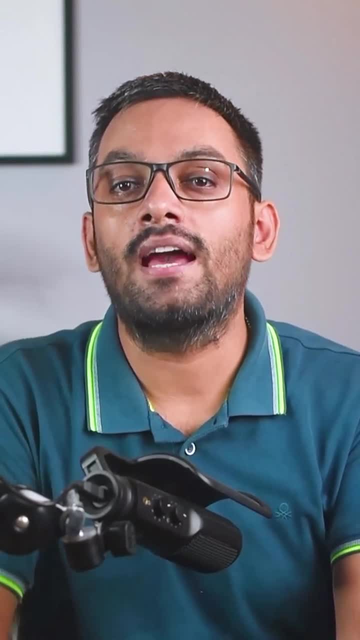 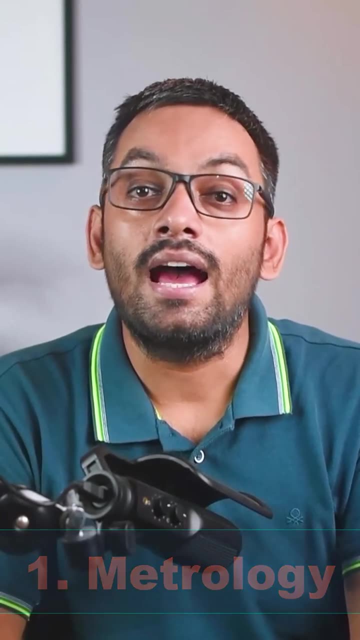 These are the three skills you should learn right now if you are a fresh mechanical engineering graduate. The first skill is metrology. It is measurement of parts and its applications, And, as a mechanical engineering graduate, you should learn to use tools like vernier, caliper. 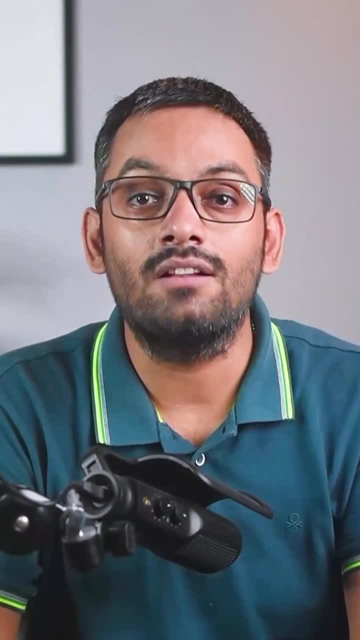 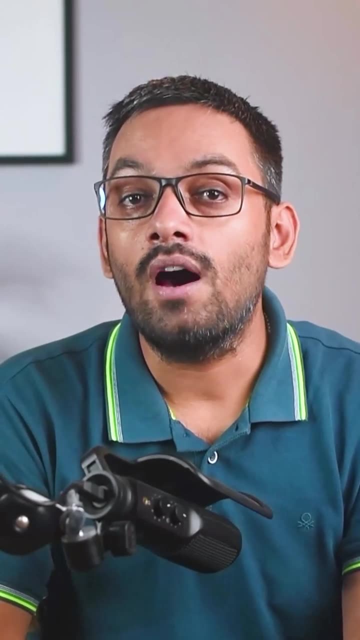 height gauge, micrometer, coordinate measuring machine and more. Now this skill will help you get the work in quality control department and it will also help you if you are involved in manufacturing of mechanical parts. Now next skill is CAD, CAM and CAE software. 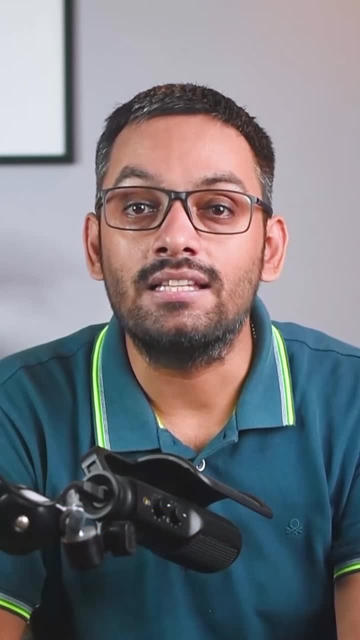 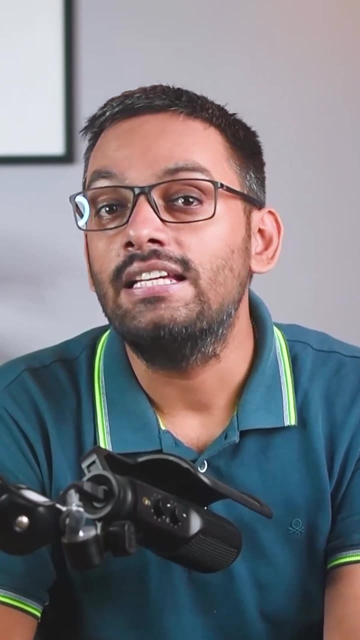 So learning to use software like AutoCAD, Solidworks and NSYS will broaden your work profile and you will be eligible to apply for a variety of positions across different skill sets. Finally, GD&T is the third and one of the most essential skill you should learn as a mechanical. 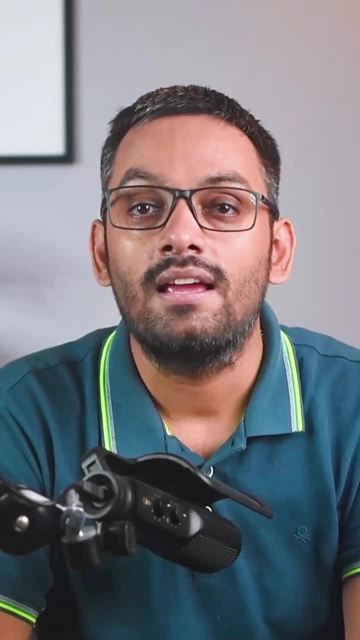 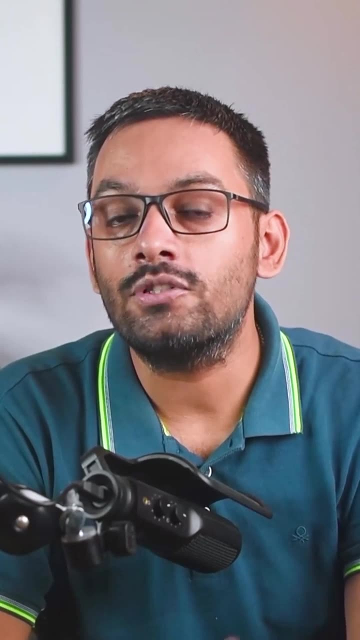 engineer. GD&T is basically language of tolerancing and it is now a required skill in several industries involved in manufacturing. So that was my pick of skills. If you want more such tips, subscribe to SourceCAD now. 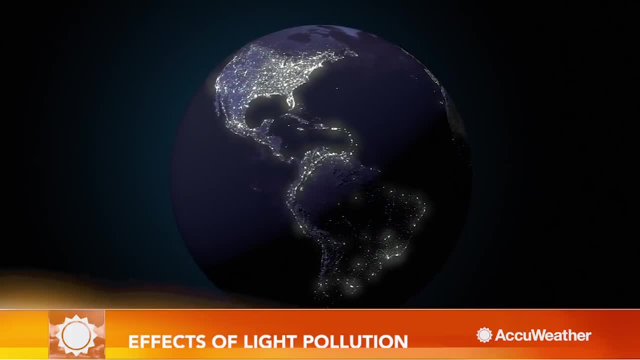 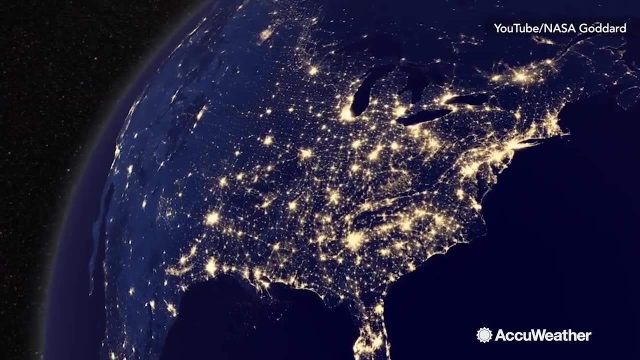 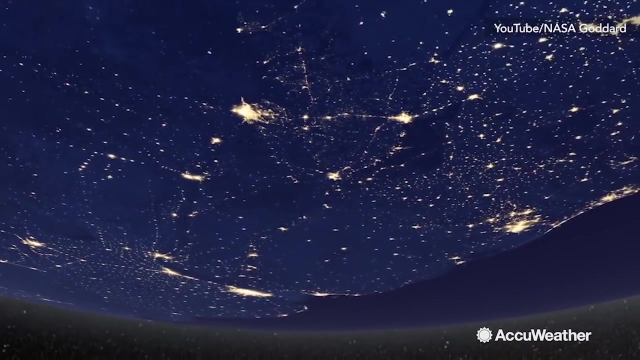 Look at any photo of Earth's night side and you see the planet lit up like a Christmas decoration. It's a unique perspective of human activity the world over. As the glowing lights of bustling cities expand, the serenity of natural darkness wanes. 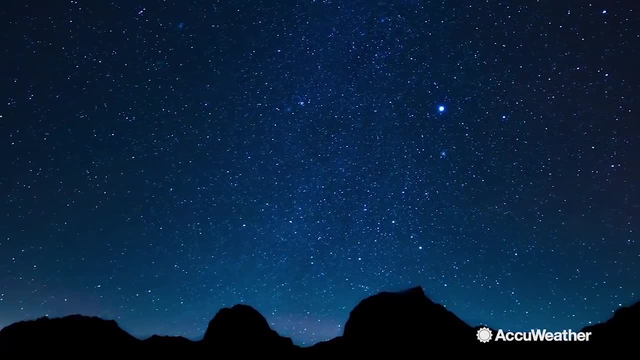 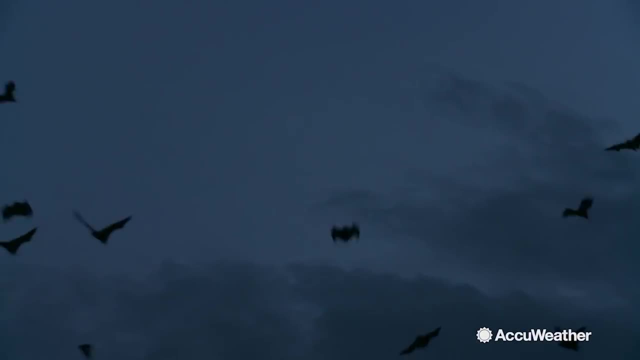 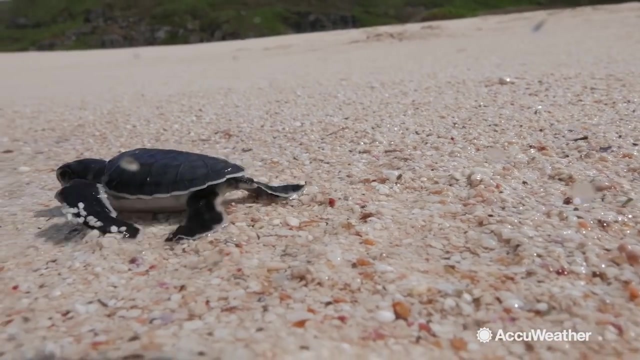 But the repercussions are not just the loss of the starry night sky. Light pollution also affects animals who depend on a nighttime environment to survive. Burnt species use the stars to navigate at night. Baby sea turtles use moonlight reflected off the ocean to guide them back to the water. 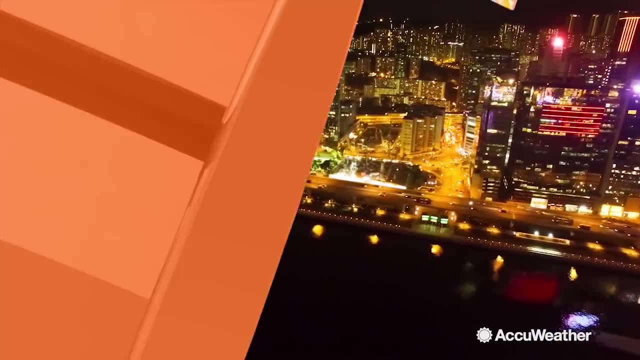 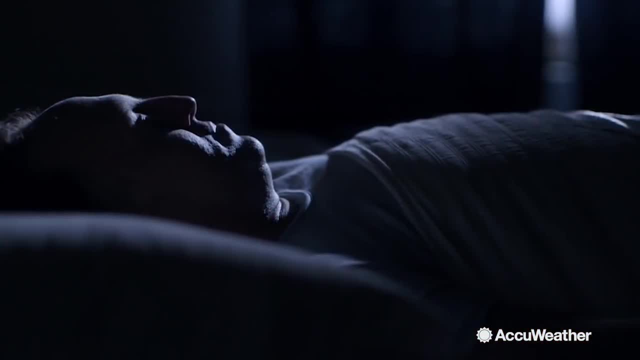 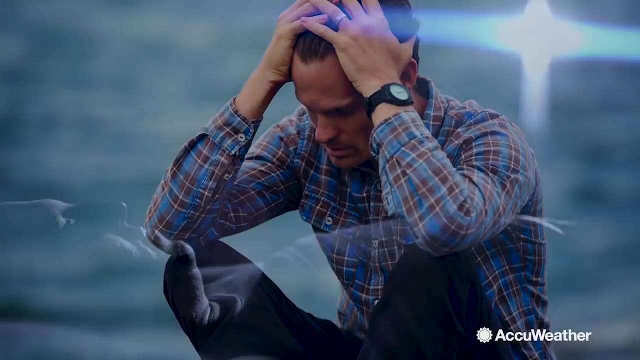 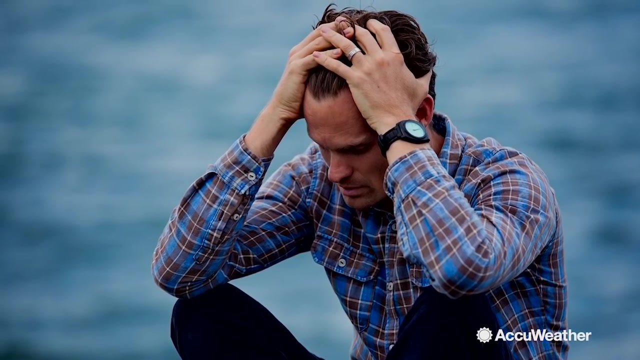 City lights can confuse them and veer them. off course, Humans are not immune either. Excessive exposure to artificial light at night can increase the risk of sleep disorders. Our immune system relies on sleep to fight against illnesses. Excessive light exposure has also been linked to obesity, depression, diabetes and even cancer.